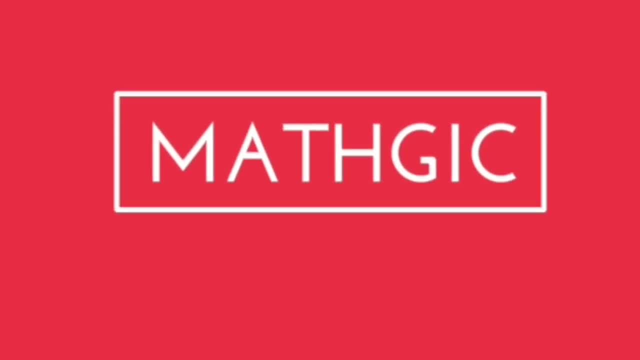 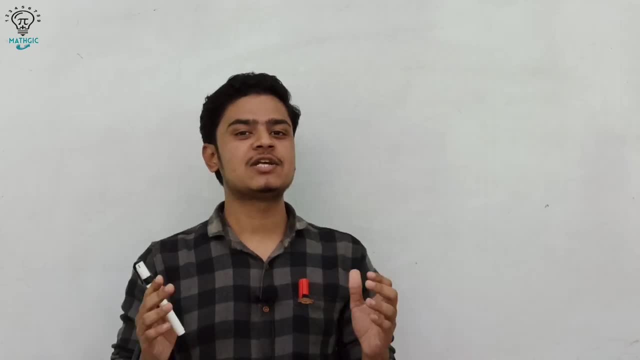 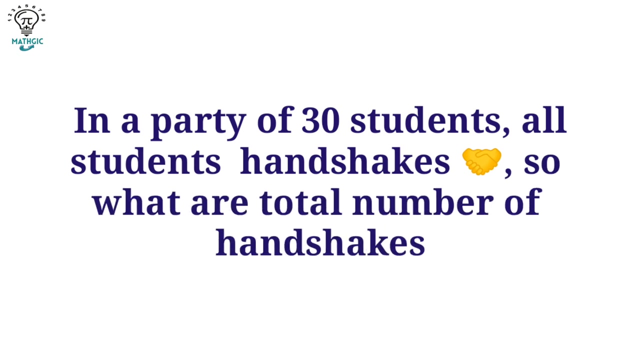 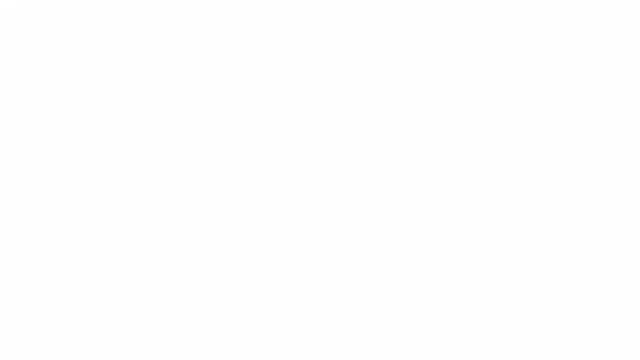 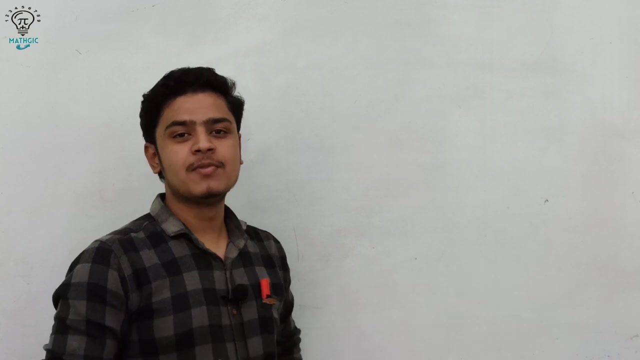 Welcome back to magic. In this video we will solve a very interesting problem. So let us first see the problem. We will solve this by two methods. So each student handshake with all 30 students but cannot with own. So where to find what are the total number of handshakes? 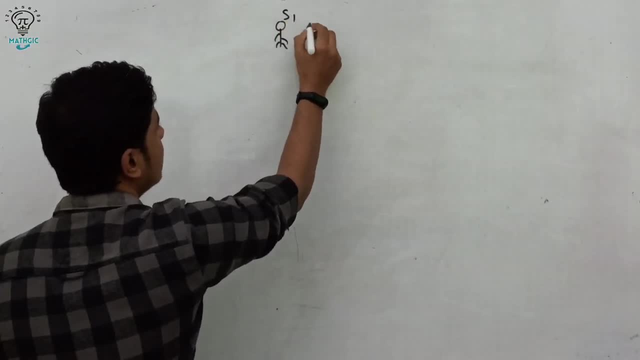 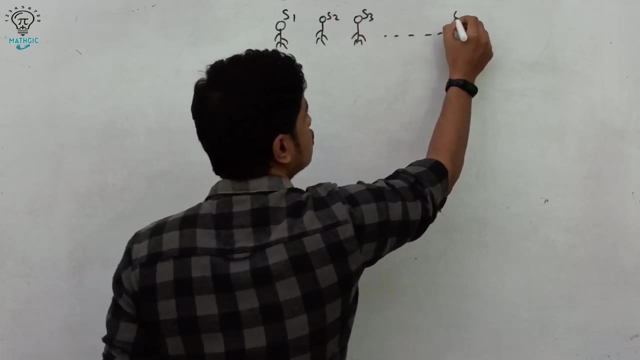 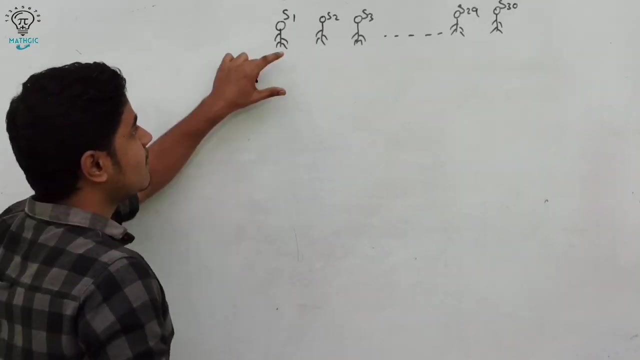 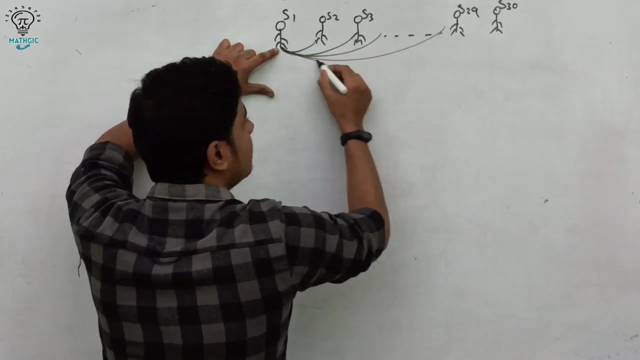 So see. So there are 30 students, Student 1, student 2.. Student 3.. Likewise student 29 and student 30. So handshake by: student 1 is student 2, student 3, student 4.. Likewise student 29 and student 30,, but cannot with own. 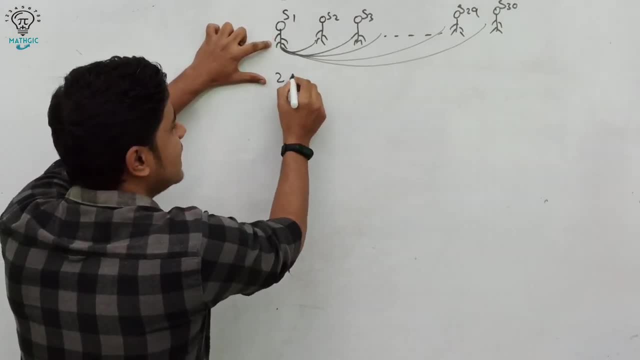 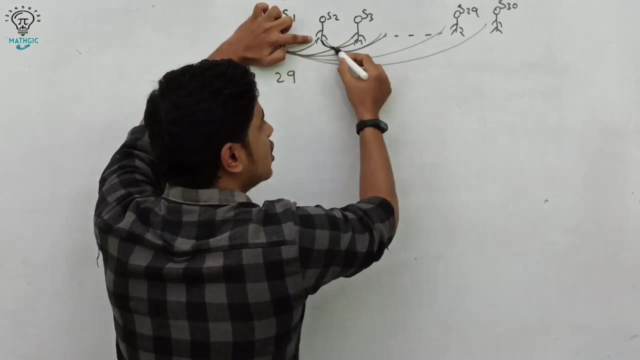 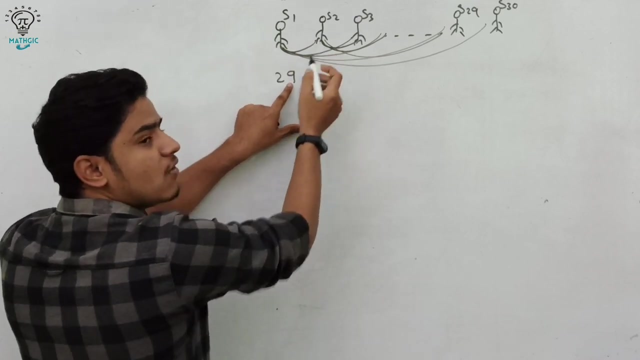 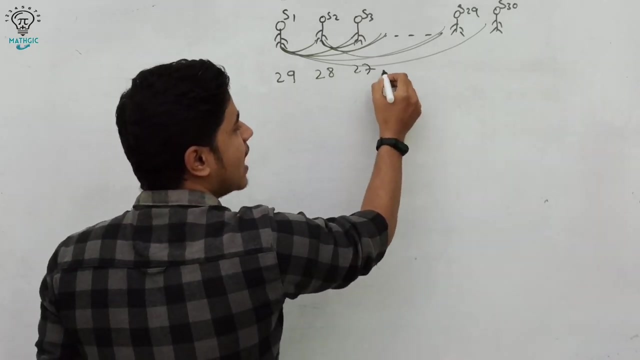 So means total number of handshake by student 1 is 29.. And similarly by student 2 is So first handshake with 3, student 3, student 4 and so on, But cannot with own And previous handshake is counted. So total number of handshake by student 2 is 28.. Likewise student 3 is 27, and so on. 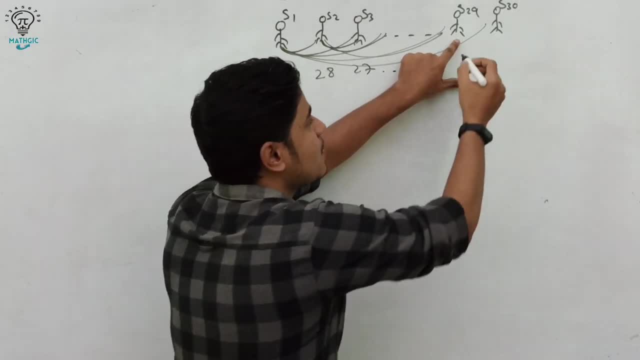 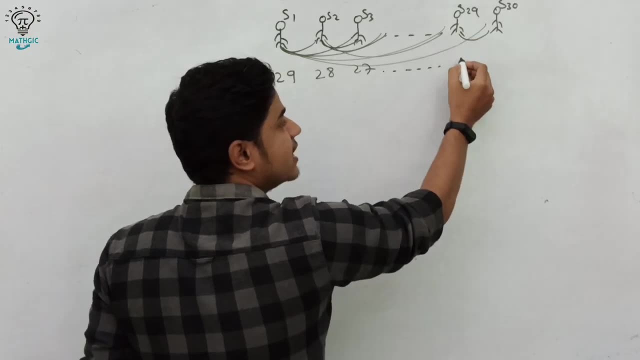 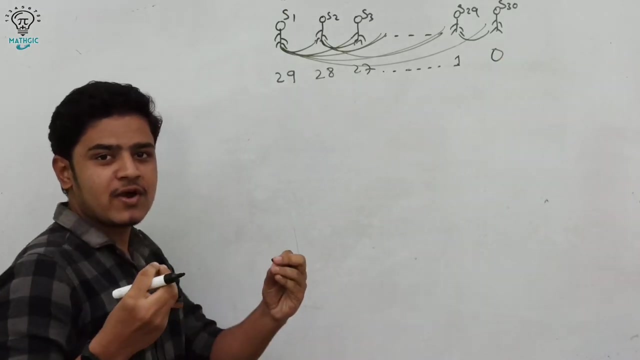 But total number of handshake by student 29 is only one because he cannot handshake with his own But previous. all handshakes are counted. So handshake by 29 students is 1.. total handshake by student 30 is 0, but we have to find total number of handshakes. So 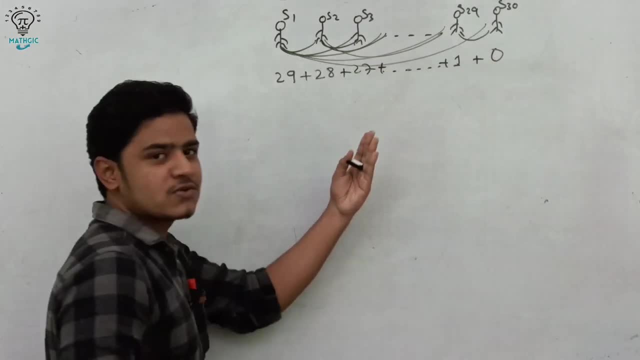 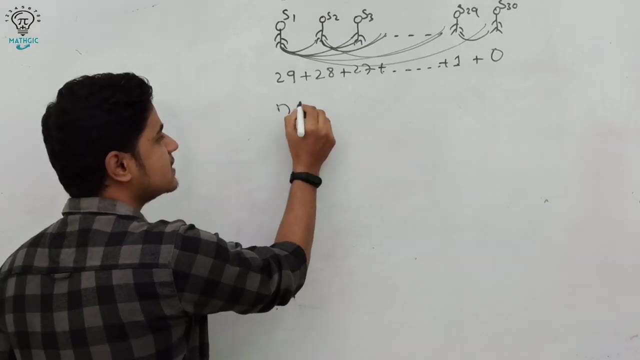 add them all. So observe the series. This look like arithmetic series, So we know how to find the sum. So there is a formula. It is n times n plus 1 divided by 2, where n is the number of. 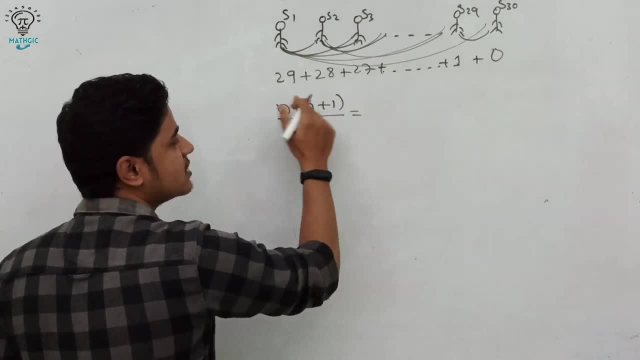 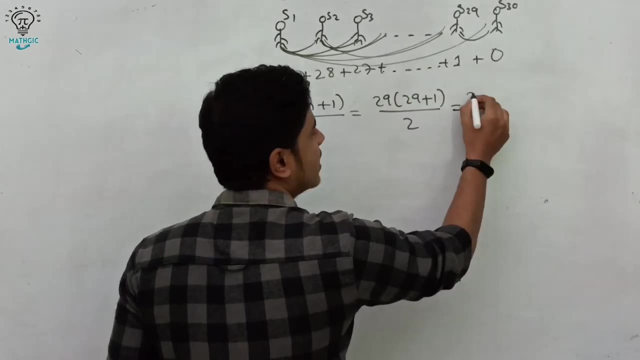 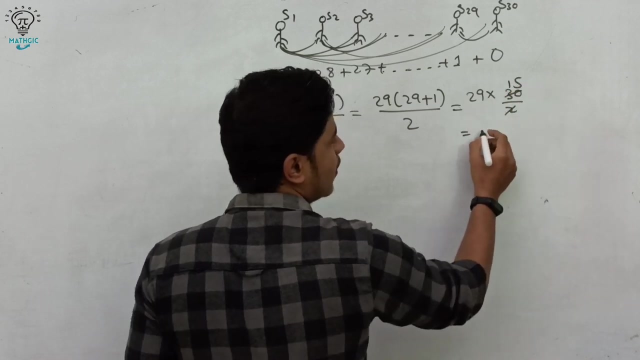 terms. So there are 29 terms, 29 plus 1 divided by 2, and 29 into 29 plus 1, 30 divided by 2.. Now half of that is 15.. 15 times 29 is 435.. So the total handshake by all the student is 435.. So